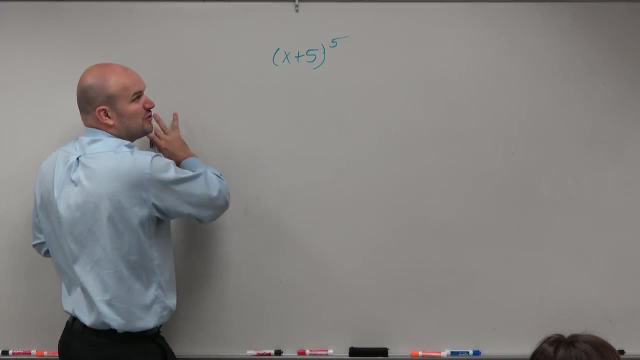 It started x to the fourth, So, automatically, what I'm going to do is I'm just going to create a set of binomials, So I know that my first term is x to the fifth, 5 to the 0, right. 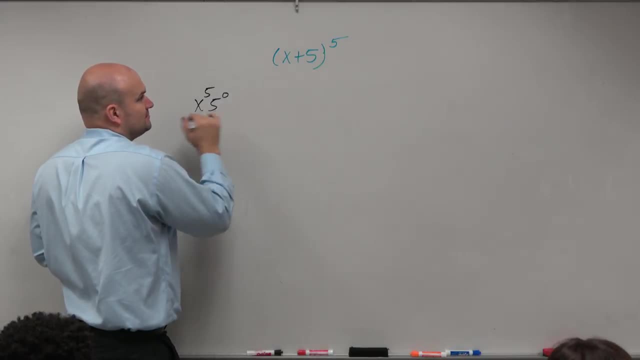 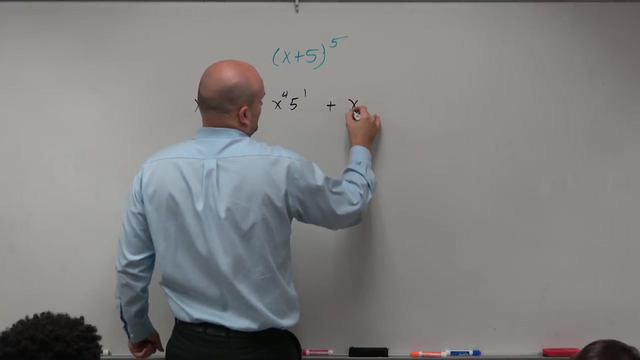 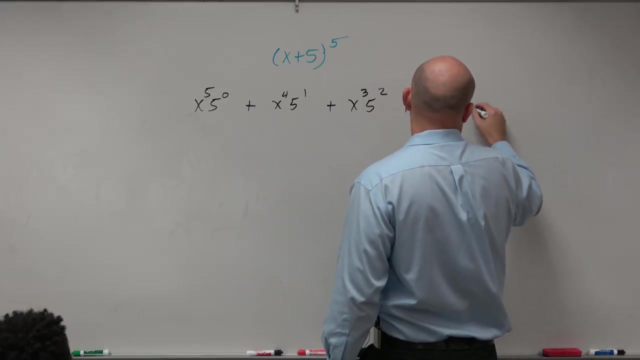 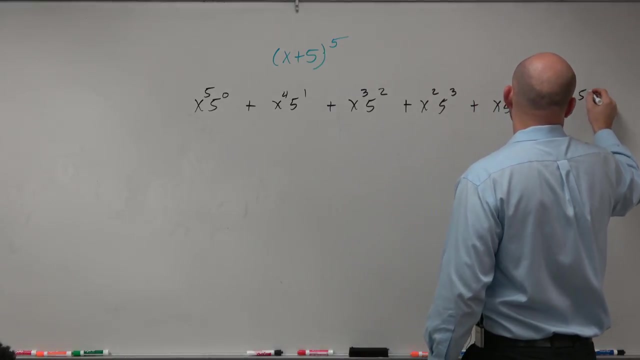 Well, we're using 5 instead of y this time. Then I'm going to have plus x to the fourth, 5 to the first, plus x- cubed, 5, squared. plus x, squared, 5, cubed. plus x. 5 to the fourth, plus x to the 0, 5 to the fifth. 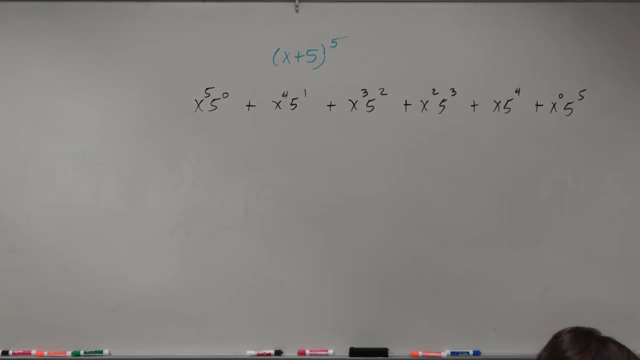 Does everybody see how I at least spread that out? All I did was the ascending descending. To me that is the easiest thing to understand. is the ascending descending. Now the next portion. and again, also remember, guys, 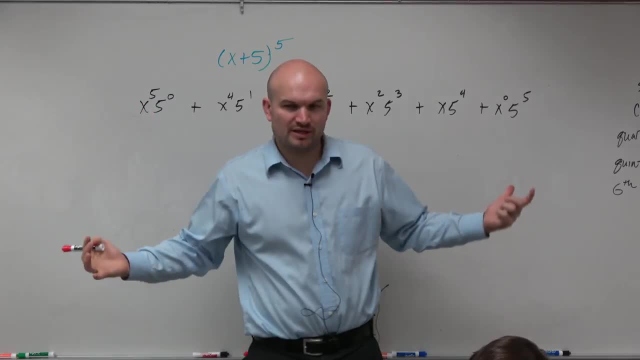 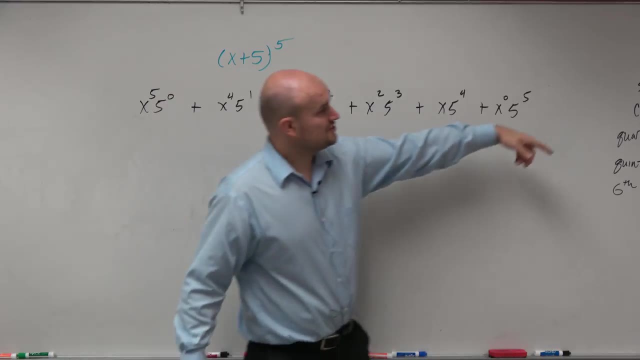 x to the 0 is 1,, 5 to the 0 is 1.. So they really don't, but I like to write them in there, so I remember this. The next example is: this is raised to the fifth power. 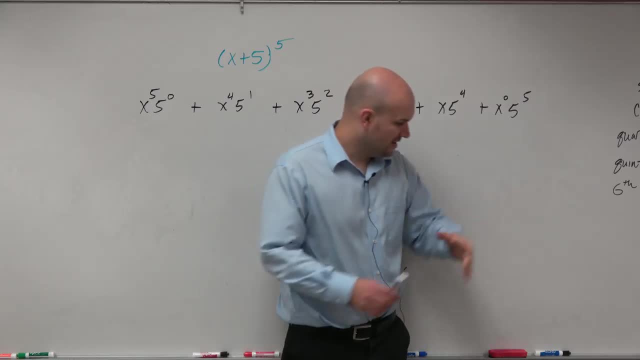 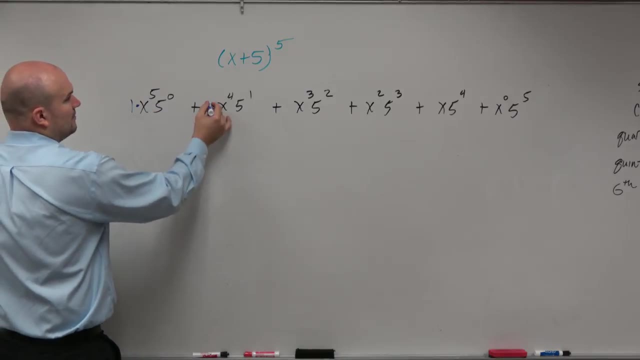 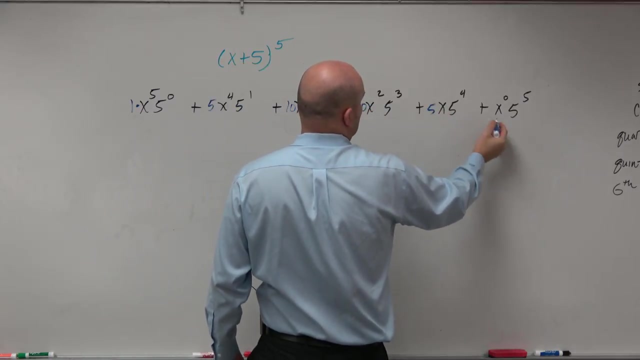 So I go down on my fifth row on the Pascal's triangle And I realize that the coefficient, the coefficients, are going to be 1,, 5,, 10,, 10,, 10,, 10,, 5, and 1.. 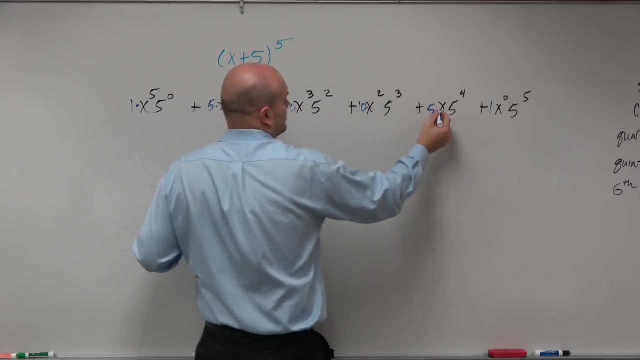 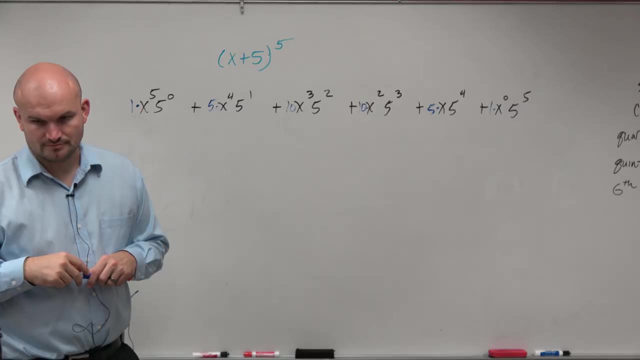 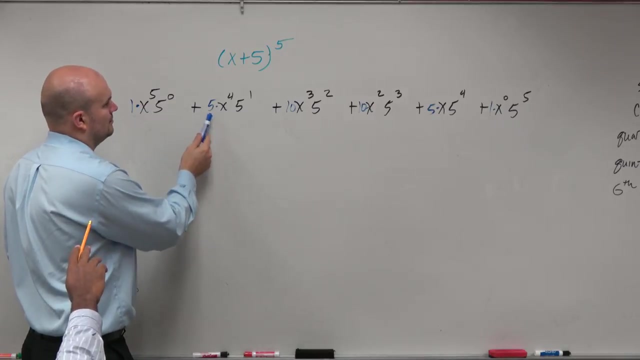 Now again, these are all multiplied. Does everybody see that? Yes, Hold on, why did you add that one in there? Yeah, Where 5 to the 0 is, Yeah, no, I haven't simplified it, though, yet. 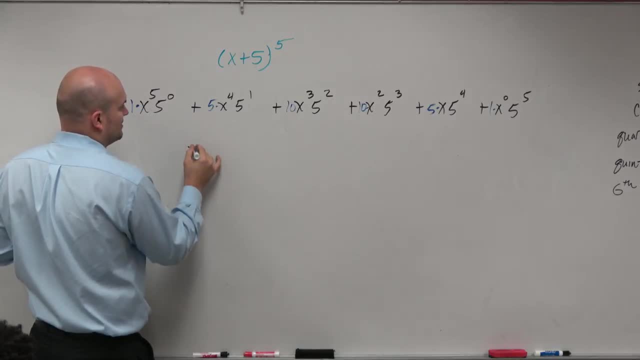 5 to the 0 is 1.. So therefore I can just rewrite this as: x to the fifth. This becomes: 5 to the first is really 5.. But 5 times 5 is 25, x to the fourth. 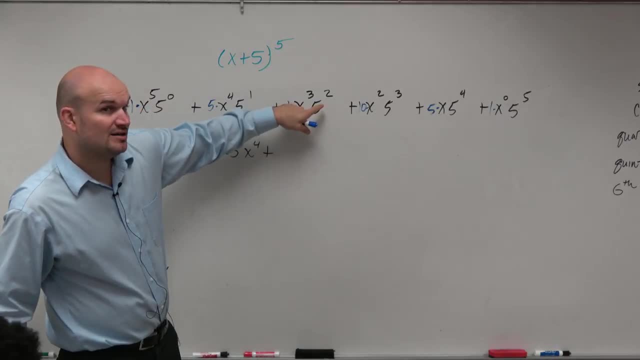 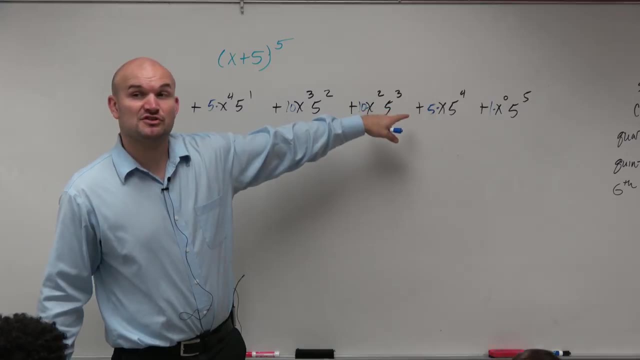 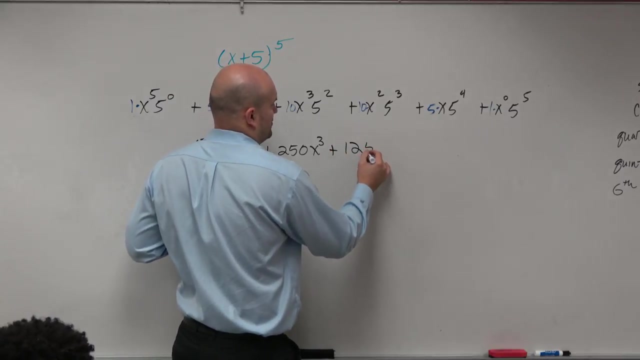 Plus, here I have x cubed. This is 5 squared. 5 squared times 10 is 250x cubed. Here I have 5 to the third power, which is 125.. Times 10, which is going to be 125, 0, x squared.